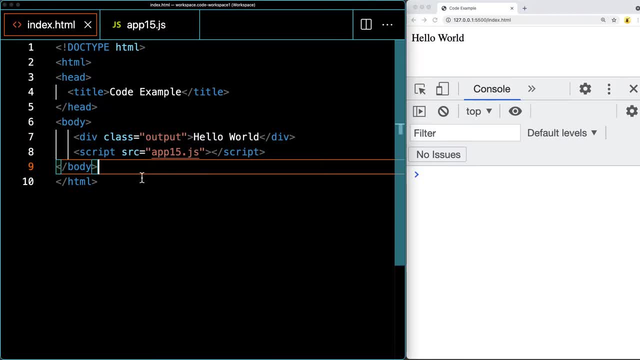 updates manipulating the style properties. I've connected it to a script source file- app15.js, opened up within the same directory as the index file. So first of all, we're going to select the element that we want to interact with, So using 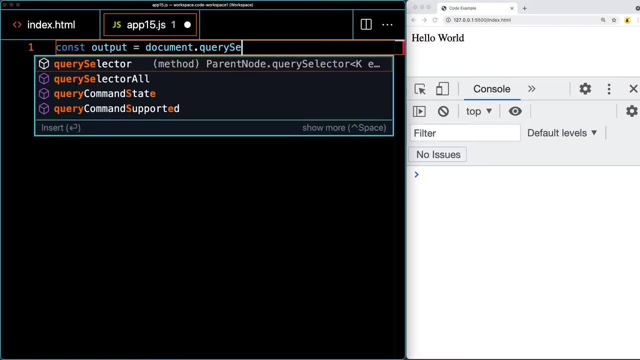 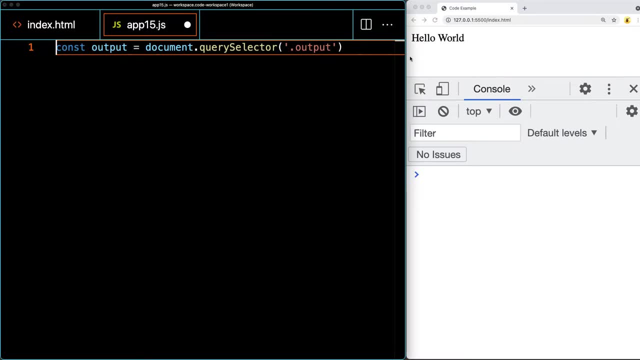 the document and query selector. let's select that element and this is the element with a class of output. And we're going to add some elements, creating them on the fly with JavaScript. So creating our first one, I'll call it div1, and I'm going to place that within the output element. So I'm going to create elements. 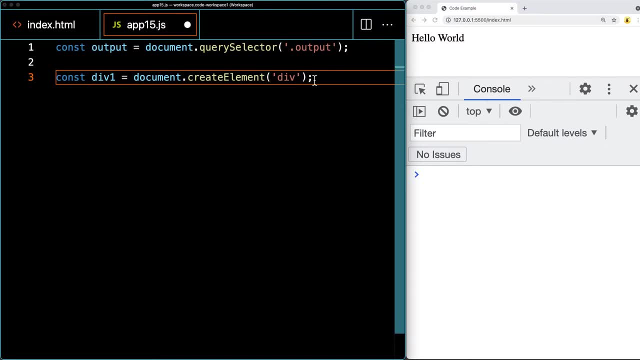 and the element that we're creating is going to be a div, And then adding that into the output and appending the element value of div1.. And let's do the same, adding in several other divs into the page, and then we'll make some updates of these elements. 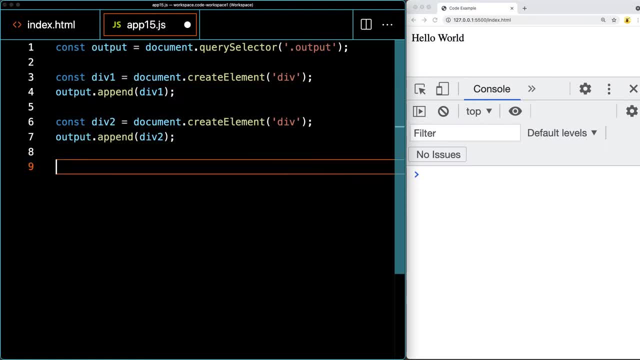 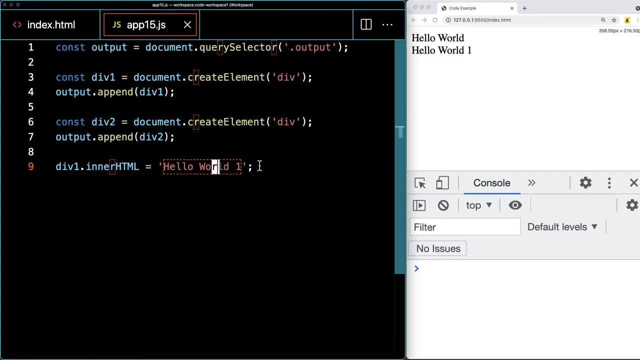 So for the first div, Tt gives us one pub 상. Now that we've got it within an object, we can add some inner HTML and that in our HTML we'll say hello world 1.. So add that to the page. 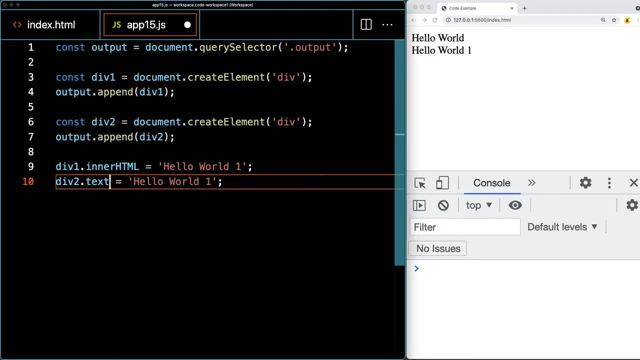 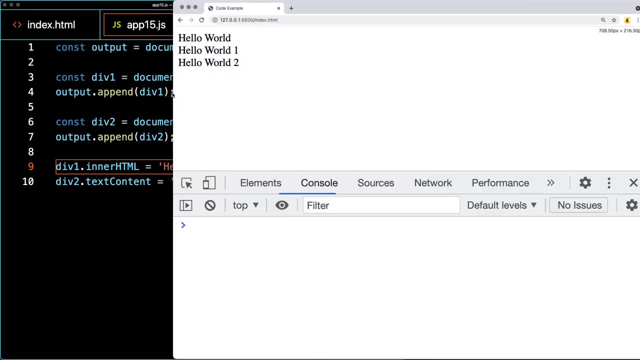 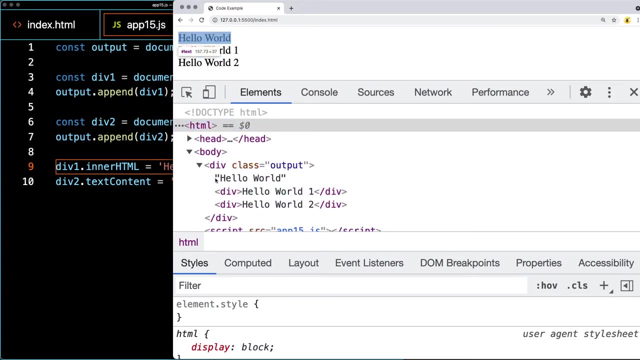 So this whole world 1 and I'll update, adding in two div 2.. And if you don't need to add any HTML text, you can just use text content to update. Uh at the element values within the source code of the elements, within output, there's our original. 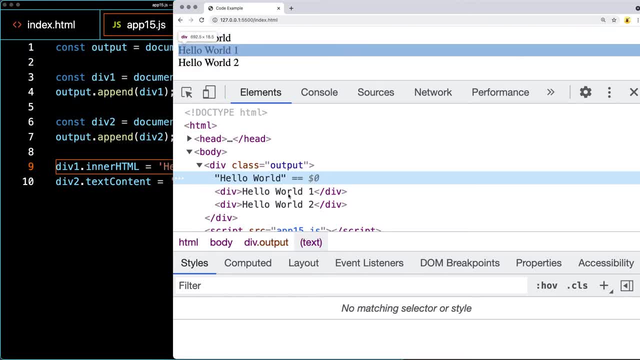 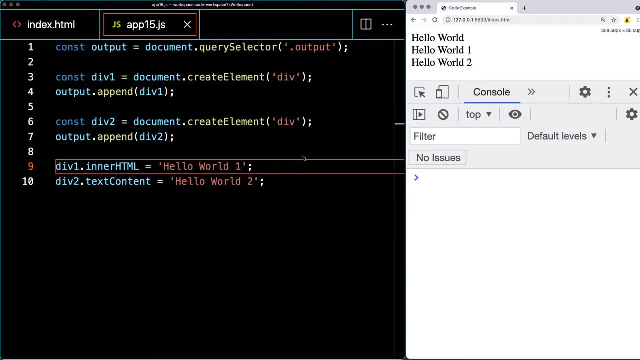 content within output and then we appended it by adding the two divs that we created dynamically with javascript code. so let's apply some styling properties to those elements and the styling can be done. so, as long as you're doing it after you've created or identified, selected the element from. 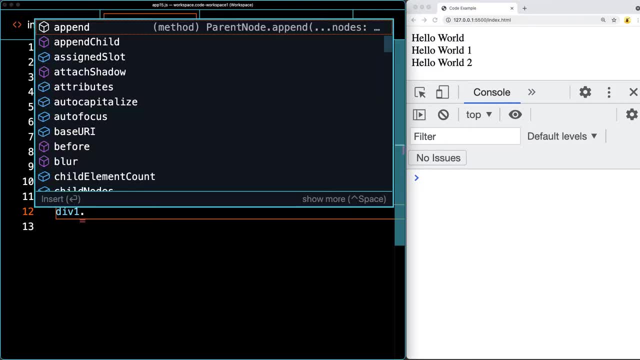 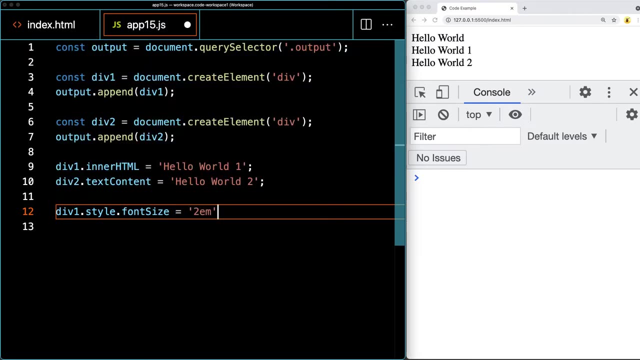 the page, then you can interact with the element object. so the styling is done with the style and within the editor. you can see there's quite a lot of options here that we have for style. there's things like the font size, and notice that it's all done within a camel case so we can set the 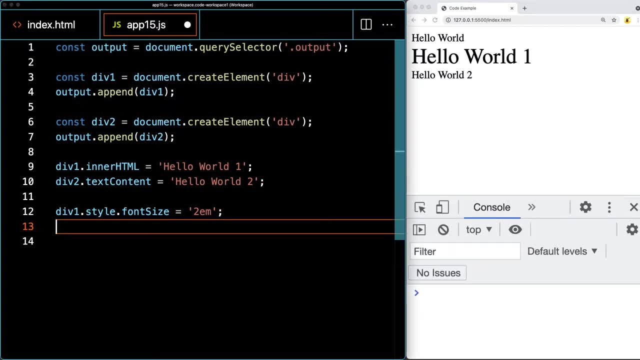 property and the value associated with that property. we can also set style, and then there's padding for the element, so we can use pittsburghcom for the padding, and actually that's going to be pretty big, so let's stick to 10 pics for the. 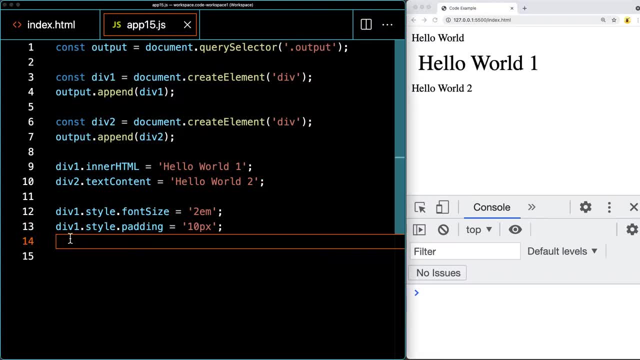 padding, so that adds in a 10 pics for padding around it. so div 1 style and let's set the border property. so the border property. we can set the individual border, so the left, right and top, or we could do for the entire border, just like we do with styling, where we're selecting and applying. 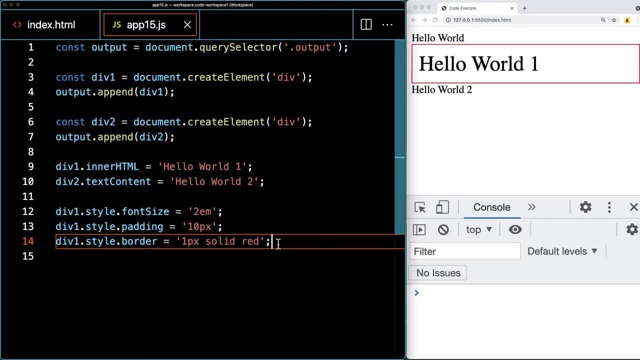 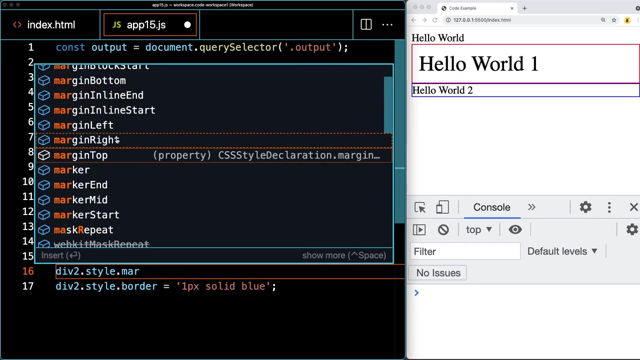 that as a shorthand method to apply the styling to the element, let's also do a border for the div 2 and for this element, setting a blue border, i'm going to add some margins for div 2, so style and margin and you can do margin top as well as left right, there's margin bottom and then there's the. 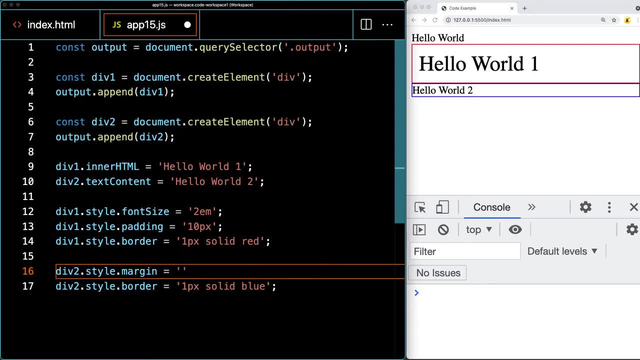 shorthand for margin for all the way around. so if you want to add the margin for top and bottom, just like with styling, we can do a 20 pics for top and bottom and then left and right. we can keep that auto, so that will automatically set the border for it. div 2 style: you can also update the width if you. 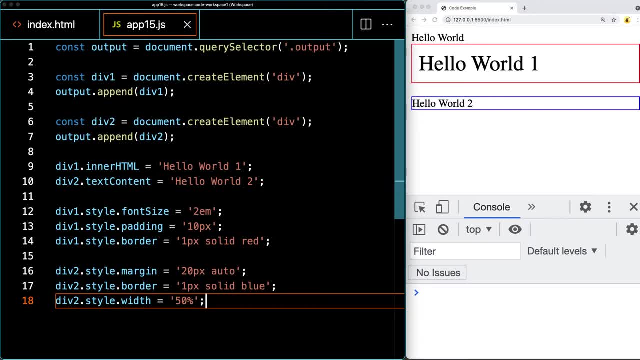 want. so the width. let's set the width to be 50 of the page and because we've got the left and right margin set to auto, that's automatically going to center it. let's also apply some styling and we'll do a text align styling, so in order to center the text. 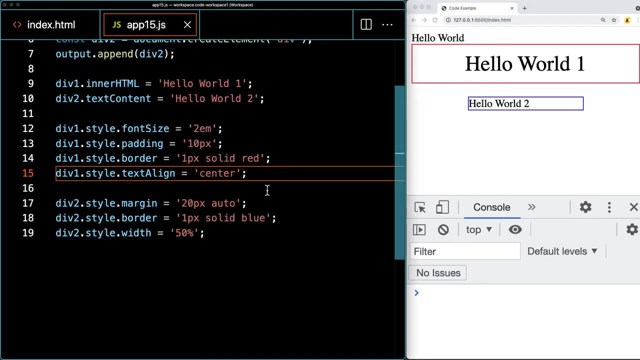 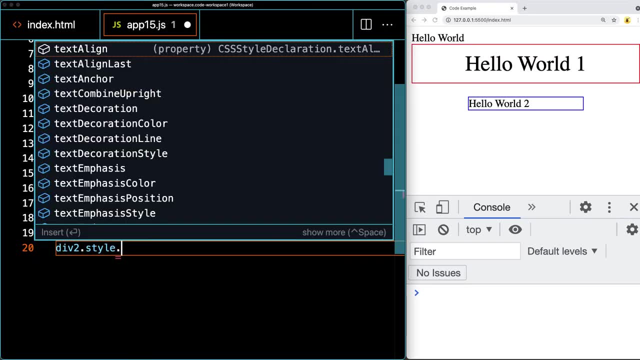 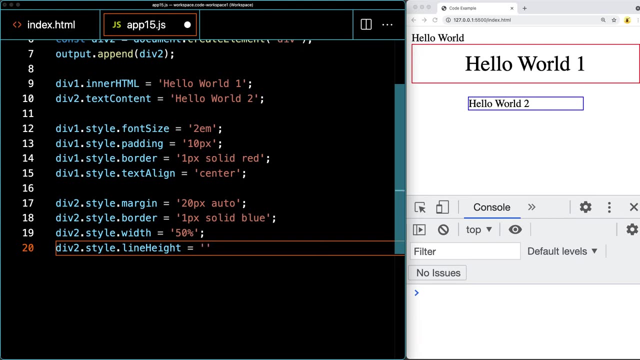 we can apply that to center the text. there's also where we can update the line height. so anything that you can do with styling, you can do an addition. so setting the line height, and i'll set the line height to be 50 pics, and then also for the element itself,